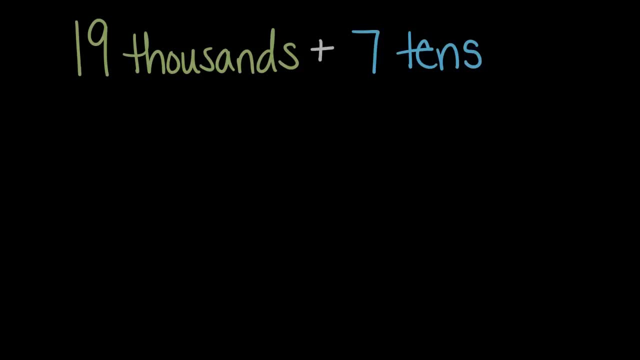 So 19,000s would quite literally be if we had 1,000 19 times. So there's 1,001 time. 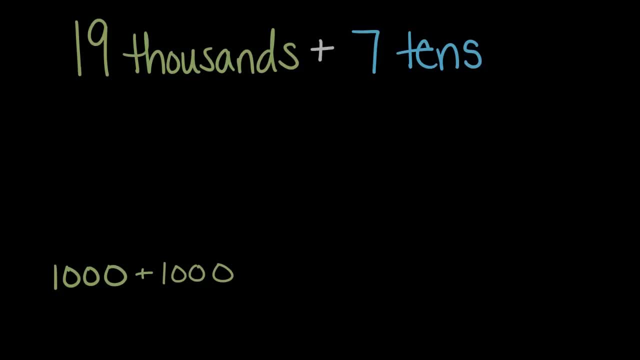 If we had 1,002 times, we would have 2,000. If we had 1,003 times, we would have 1,000, 2,000, 3,000. And the pattern here should be pretty clear. 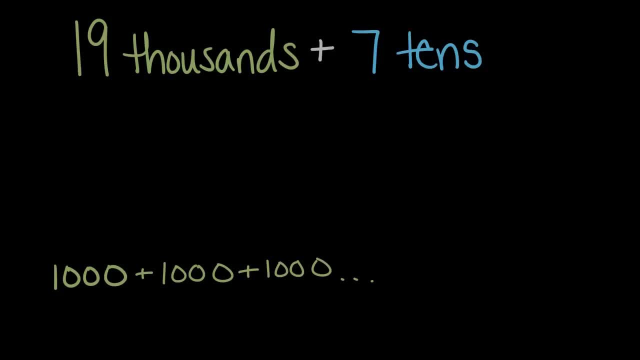 If we had 19,000s or 1,019 times, we would have 19,000. 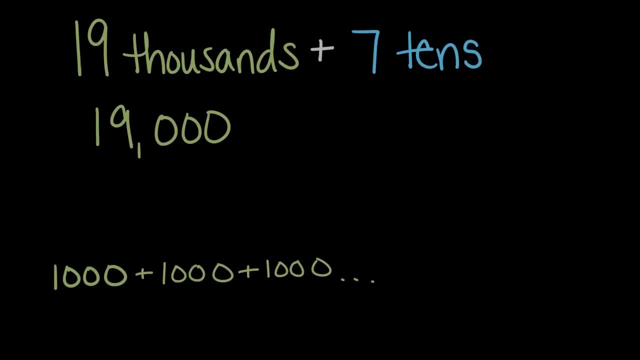 So 19,000s is literally 19,000s. And then seven 10s, same thing. We could have seven 10s, we could have 10 seven times. So 10 plus another 10. And this one's a little simpler to do than the 19. We only have to list seven 10s this time. That's six 10s and there are seven 10s. So seven 10s would be literally seven 10s. 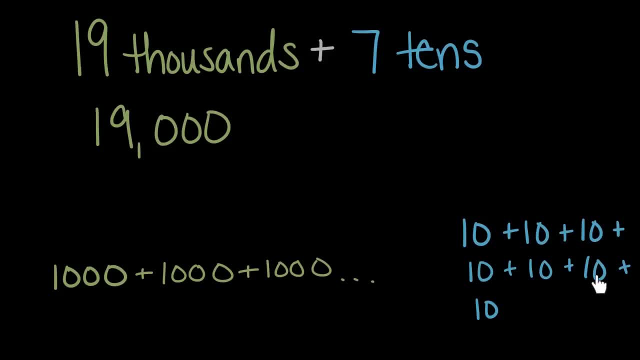 Or 10, 20, 30, 40, 50, 60, 70. So seven 10s is 70. 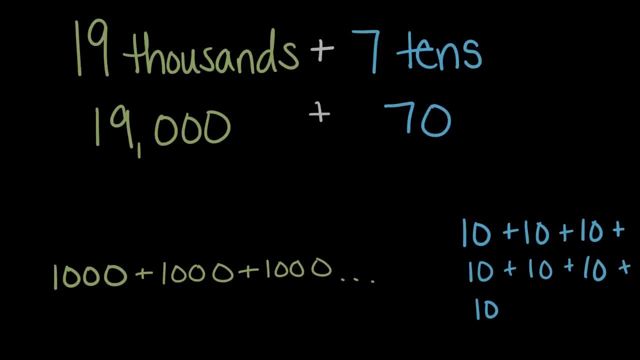 And then if we wanted to combine these or add these, we would have 19,000s. 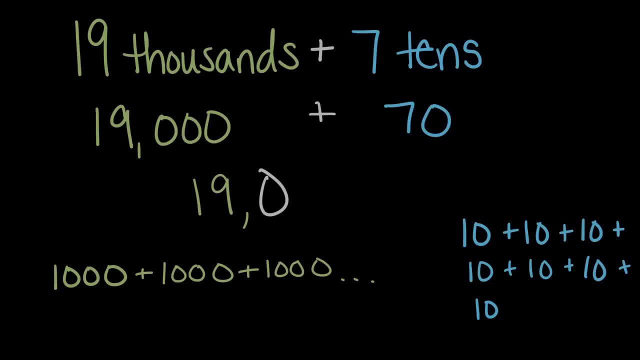 Zero hundreds, the seven 10s, and zero ones. Or 19,070. 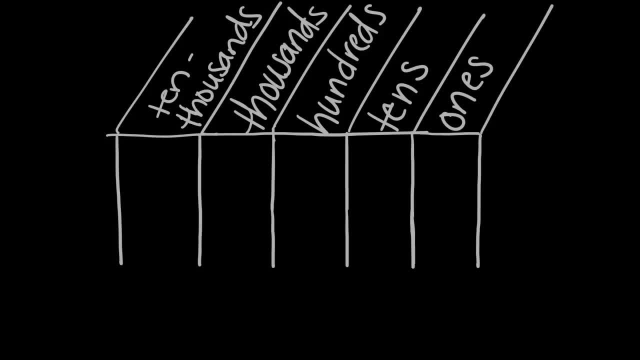 We could have also thought about that question in terms of place value. Instead of listing out all the thousands and listing out all the 10s, we could have thought of the place values. 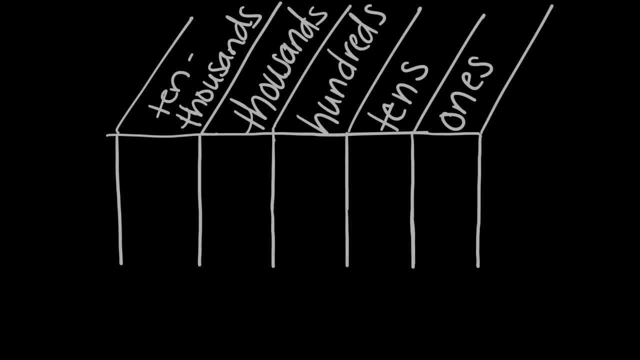 We had 19,000s, which means we want our last digit, the nine, to be in the thousands place value. So we could have also thought about that question in terms of place value. Instead of listing out all the thousands and listing out all the 10s, we could have also thought about that question in terms of place value. And then the other digit we had, one, would go in front of it. 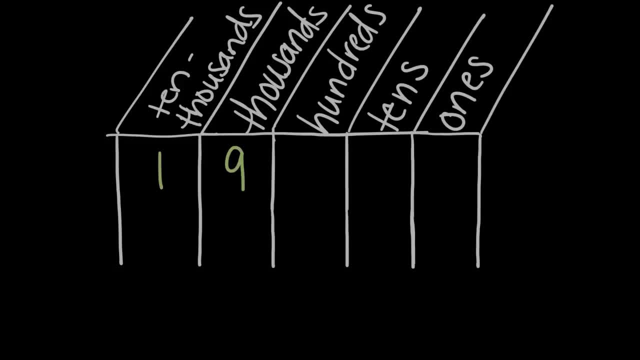 So this is red, 19,000s. And by writing that thousands there, we covered all these empty place values. 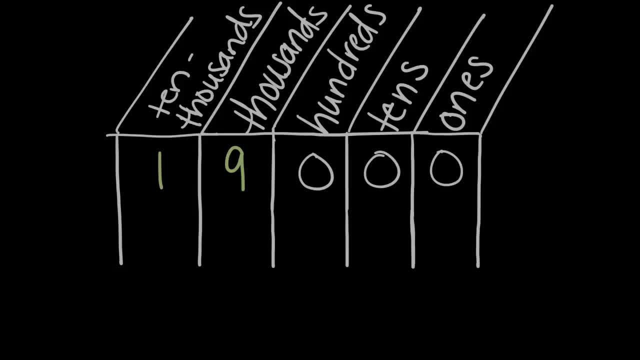 Or the three zeros we ended up adding. The thousands can be represented by these three zeros at the end. 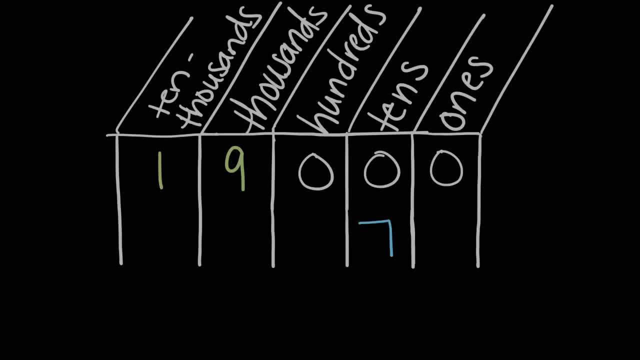 Whereas seven 10s, we put a seven in the 10s place. And again, we have an empty place. And again, we have an empty place. And again, we have an empty place value behind it. We had no ones with it. The 10s, by saying 10s, we implied this zero after it. 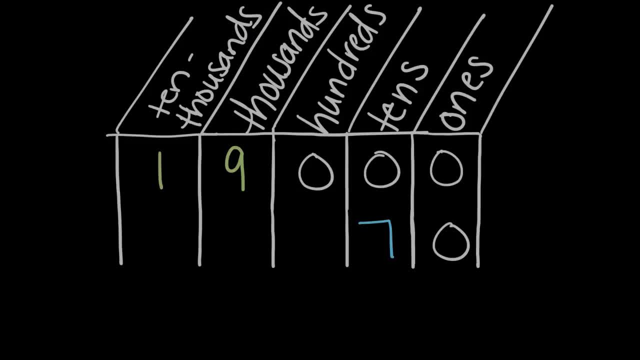 So the thousands added these three zeros to the end. And seven 10s added one zero to the end. 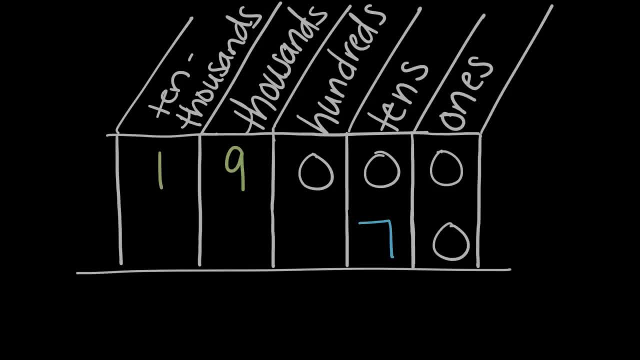 And again, if we combined them, like we saw on the previous one, we'd have 19,000, zero hundreds, and seven 10s. So either way, whether we list out what 19,000s is literally with 19,000s, or seven 10s literally, 10 seven times, or we look at it in terms of place value and add the zeros on the end, either way, our solution will be 19,070. 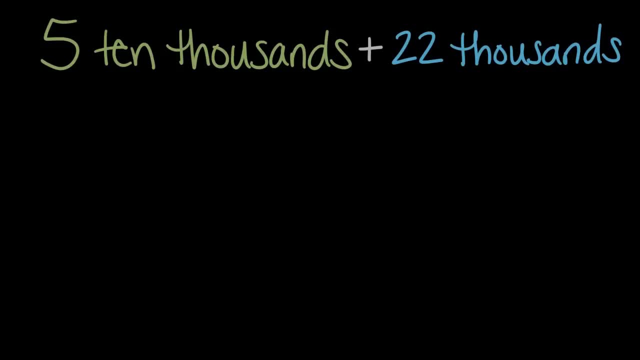 Here's one more. We have five 10,000s plus 22,000s. So two ways, again, we could try to solve this. One, we could think about what all of these zeros are. 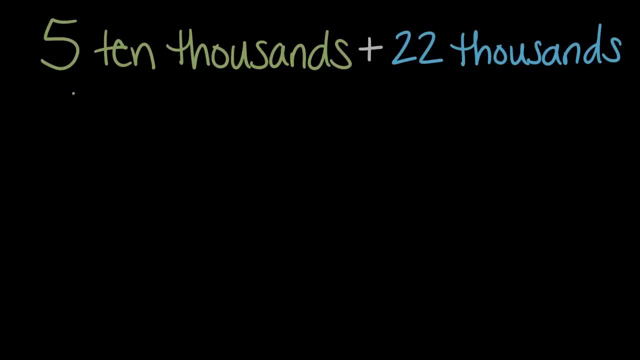 What are five 10,000s? If we had 10,000 five times, another 10,000, another, that's three, four 10,000s, and five 10,000s, that would be a total of 50,000. 10,000, 20, 30, 40, 50,000. 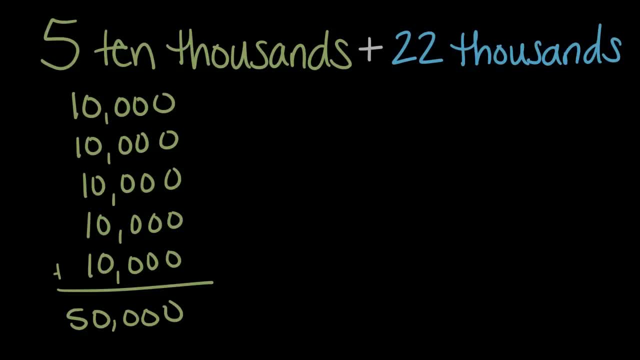 So five 10,000s is 50,000. Let's write that up here. 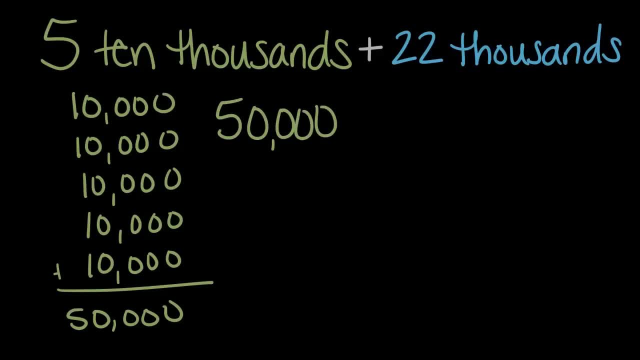 50,000, plus 22,000s, 22,000s. 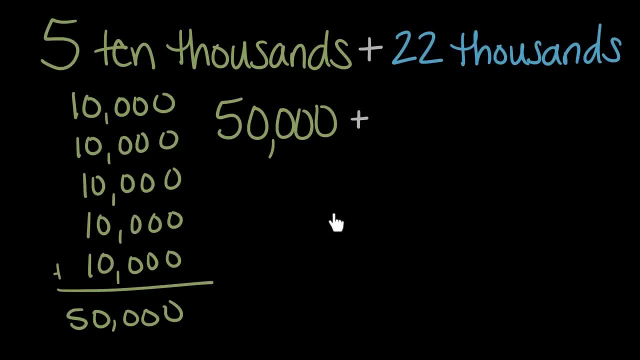 Remember when we did the 19,000s, if we wrote one 1,000, it would be 1,000. If we wrote 1,000 two times, it would be 2,000s. If we wrote it 22 times, then it would be 22,000s. There would be 22,000s. And we could combine these numbers. 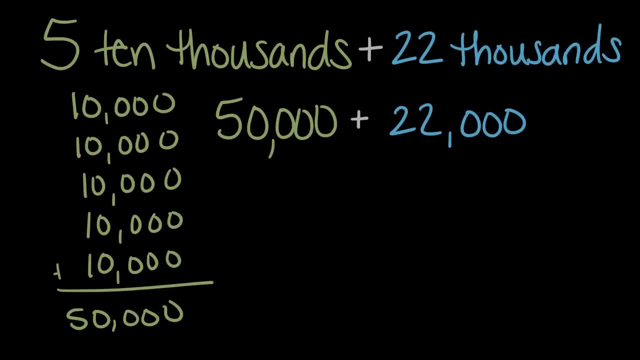 50,000 plus 22,000 will be a total of 72,000.